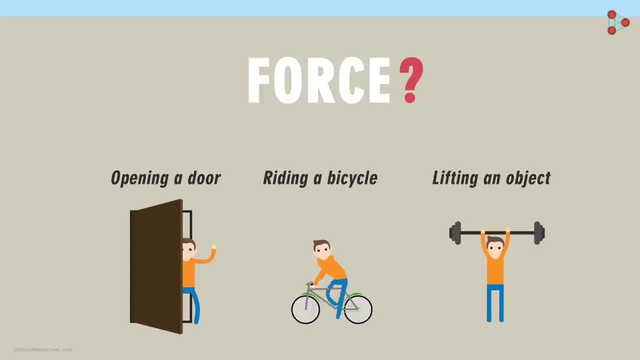 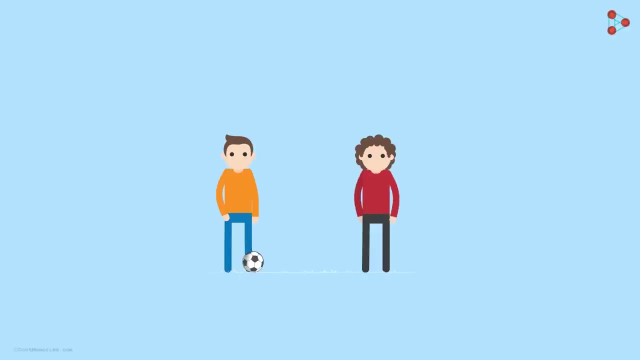 force. What is a force? Consider a ball lying on the ground at rest. It's not moving. Okay, Suppose this player here wants to pass this ball to his teammate who's standing on the other side of the pitch, How will he do that? He needs to make this ball move in. 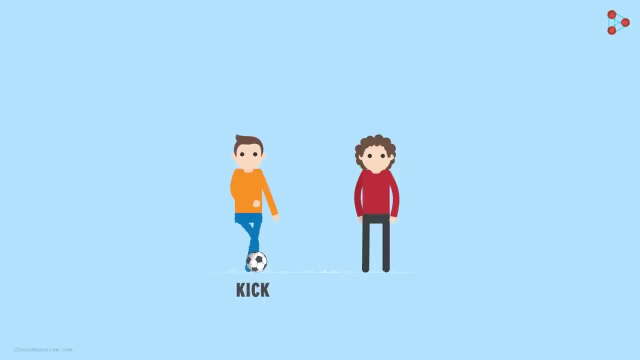 the direction of his teammate. So he will kick the ball in the direction of his teammate. When he kicks the ball, we say that he applied a force on the football. Yes, the kick is nothing but the force he applied on the ball. Now suppose that we have a desk here at point. 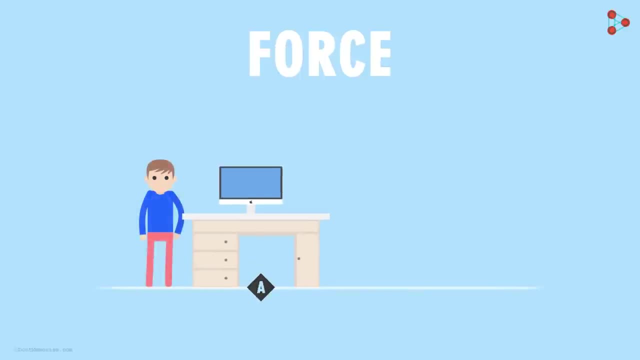 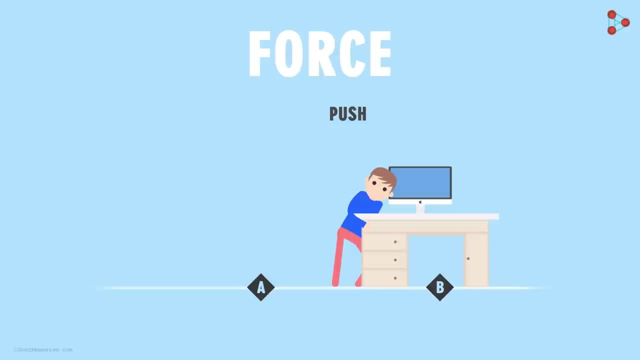 we say that the person applied a force on the desk in order to shift it. The push here is the force that the person applied on the desk. Similarly, when you lift some object from the table, we say that you applied a force on that object. Here the force is applied. 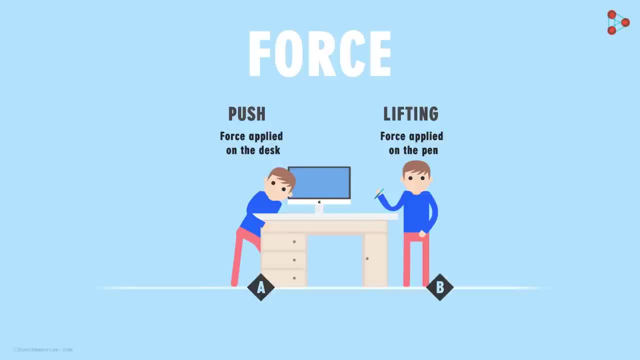 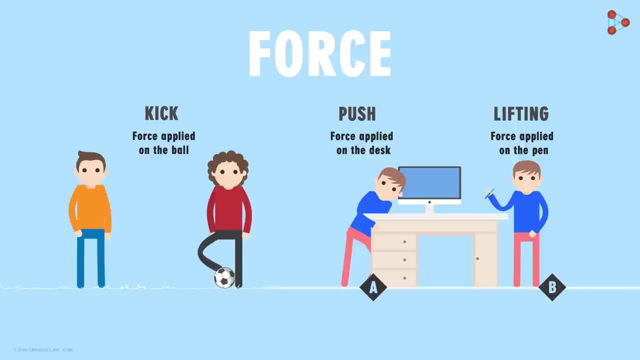 in the form of lifting. So forces are nothing but actions such as kicking, pushing, lifting, etc. performed on objects. There are many such actions that we can perform. We have already seen few of these. Some more of them are given below. 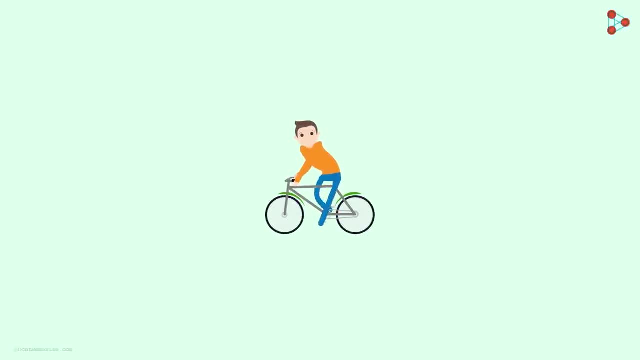 While riding a bicycle, we pedal it continuously to keep it in motion. Here, pedalling is the force that we apply on a bicycle. Hitting the hammer on a nail is also a force applied on the nail. What about stopping a moving ball? 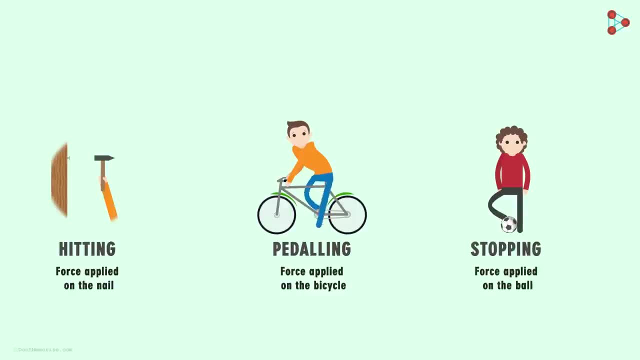 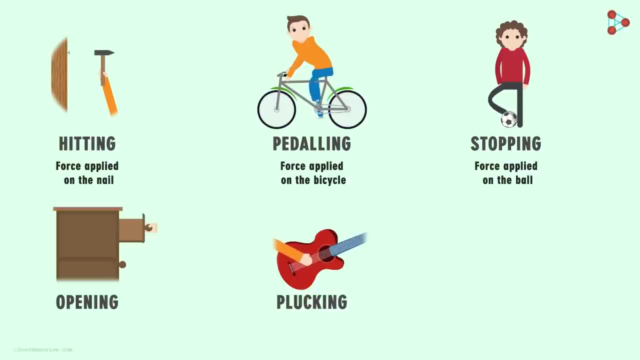 Yes, even stopping the ball means we are applying a force on it. We applied some force to stop the ball. Opening a drawer, plucking the string of a guitar, moving a piece on a chess board are some of the other actions performed on objects. 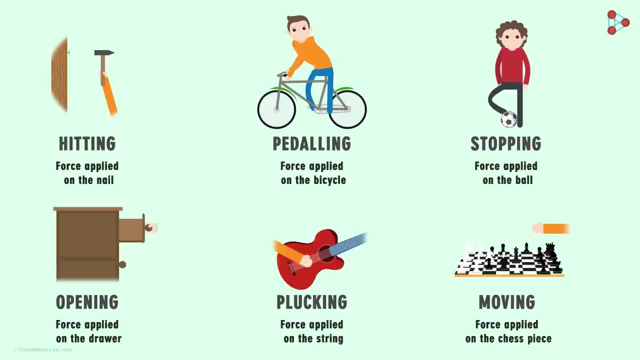 So performing these actions on objects is nothing but applying force on them. But these are just a handful of simply too many actions that we can perform on the objects, And it's not possible to write each one of those. But we can categorise all these actions into two basic ones. 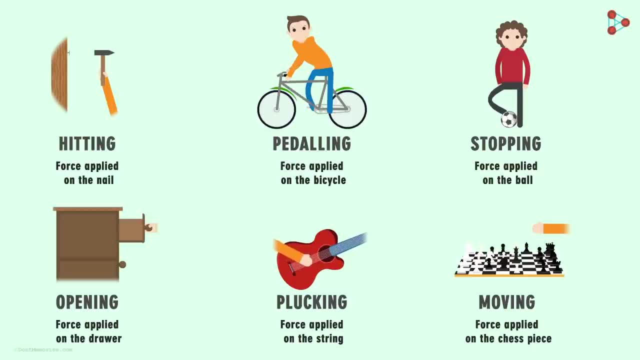 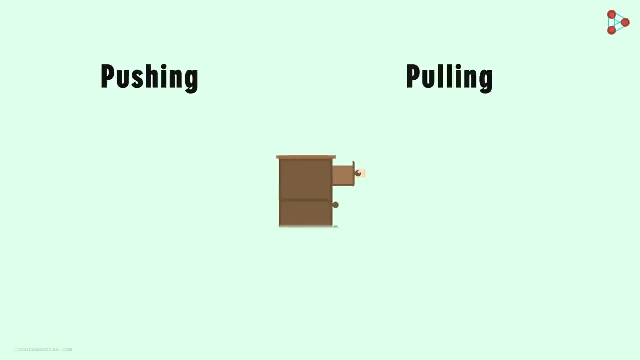 That is, we can describe all these actions under two actions, namely pushing and pulling. For example, when we open this drawer, we are simply pulling the knob of the drawer to open it. Similarly, when we are drawing or lifting a bucket of water from the well, we are pulling. 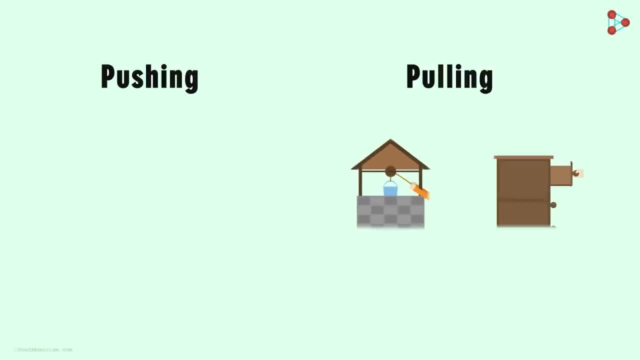 the bucket towards us. What are the actions that can be described under pushing? Actions such as passing the ball, hitting the hammer on the nail, etc. can be thought of as pushing an object. Are there any actions that can be described under both? 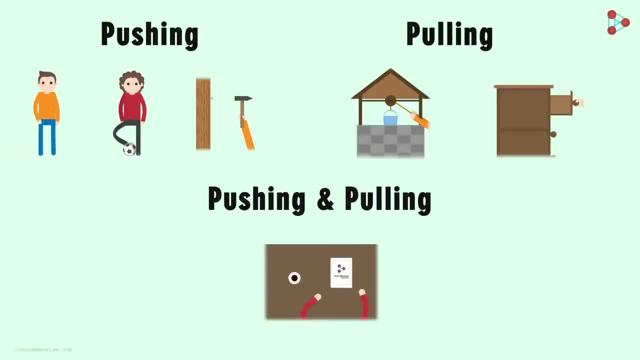 Yes, there are. Suppose there's a book on the table, you can either pull it towards you, like this, or push it away from you, like this. So moving an object can be described under both. Opening or shutting a door can be thought of as both. 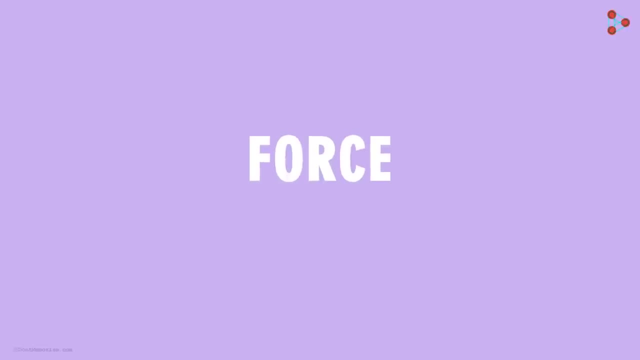 So we can safely say at this point that the forces are nothing but the push or pull applied on objects. Forces are due to interaction between the bodies or objects. What does it mean? Let's go back to our first example of this video Here. in order to pass the ball to his team-mate, the player must move it. 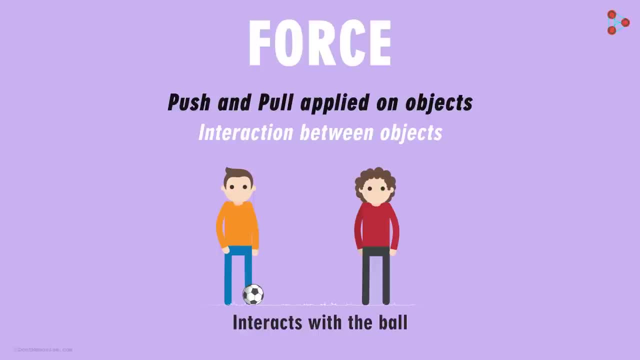 That is, he must interact with the ball to move it. That is, he must interact with the ball to move it, To move it in the direction of his team-mate. He interacts with the ball by kicking it. The ball and the player interact with each other. 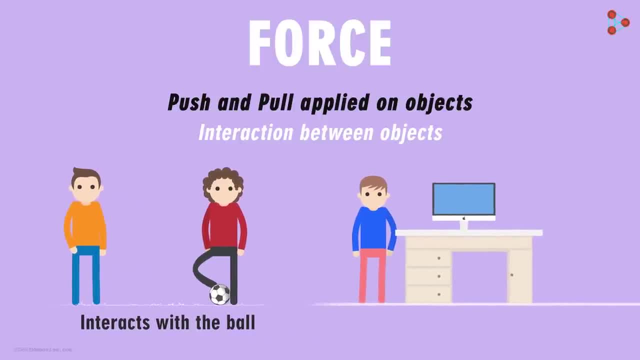 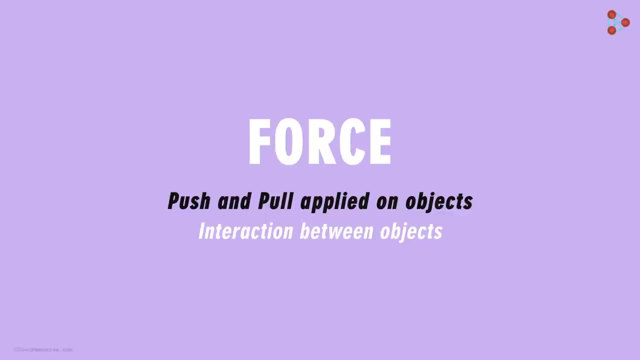 In the second example, in order to move the desk from point A to point B, he must interact with the desk. We will study more on these interactions in the future videos. Now, since we are clear with the basic understanding of what force is, let me put its definition. 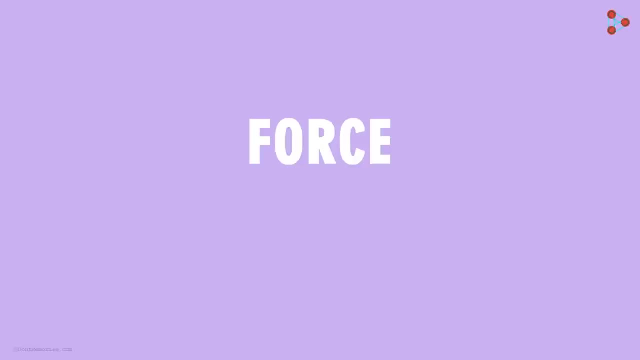 in front of you. It states that a force is a push or pull upon an object resulting from the object's interaction with another object. In the next lesson we will talk more about these interactions. See you then.